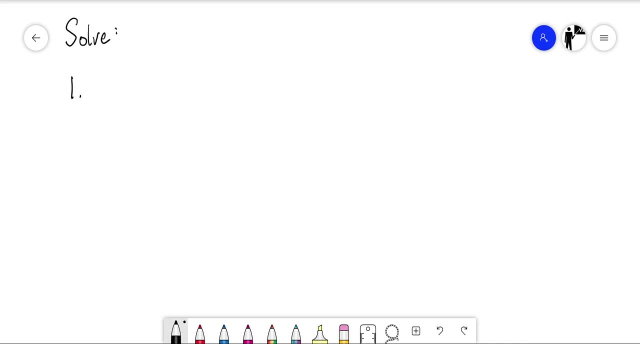 Okay, we're going to have a look at solving a few equations involving the binomial coefficient. So example one we're going to solve: n choose 2 is equal to 6.. Okay, so essentially we want to work out that if we're choosing two things from something, there's six possibilities. 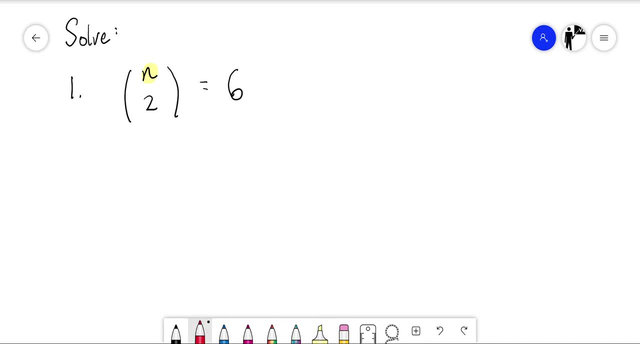 what is that? something that we're choosing from. So what we're going to do is we're going to rewrite this term here. okay, because in your formulas you're given the formula n- factorial over r. factorial over n r times n minus r factorial. So we're going to rewrite. 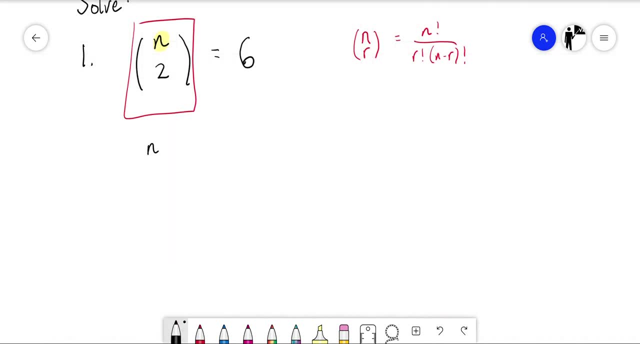 this left-hand side. So this left-hand side will become n factorial over 2 factorial times n minus 2 factorial and that is still equal to 6.. Remember, just when we think about generally, about a sequence of numbers, numbers would go n, n plus 1,. 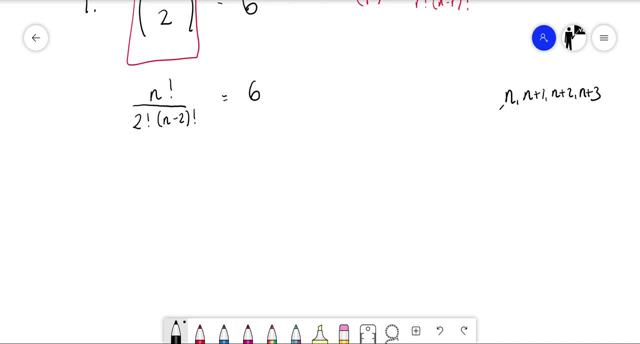 n plus 2,, n plus 3, and if we're going back the other way, n minus 1,, n minus 2.. So remember before, if we had something like 7 factorial over 5 factorial, we would rewrite our 7 factorial. 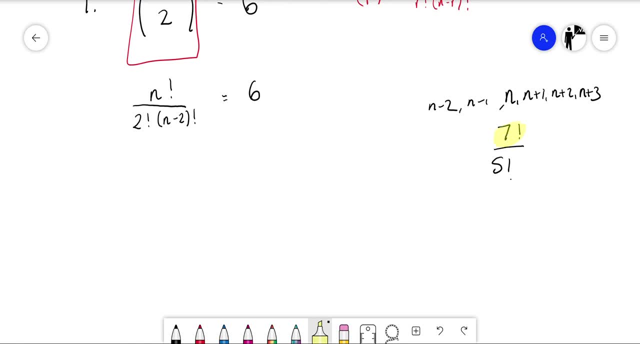 We would rewrite our 7 factorial in terms of 5 factorial. So what we're going to do here is we're going to rewrite this term here and we're going to write this term here and we're going to rewrite n factorial in terms of n minus 2 factorial. okay, So that is going to become. 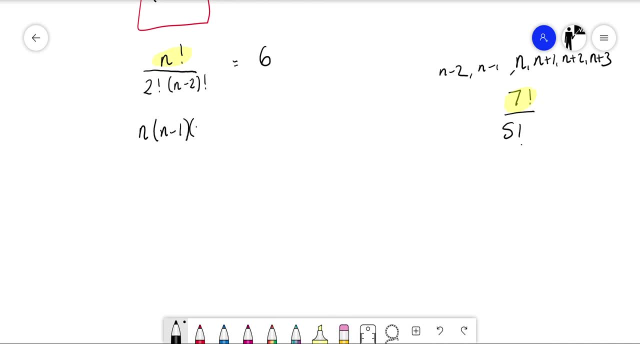 n times n minus 1 times n minus 2 factorial, and that's over 2 factorial. n minus 2 factorial, and that is equal to 6.. We can simplify our n minus 2 factorials, So we're going to have n. 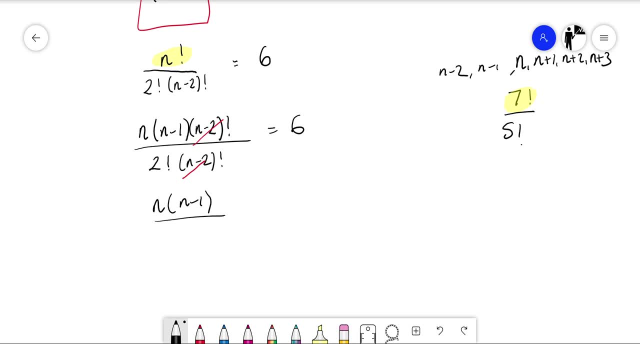 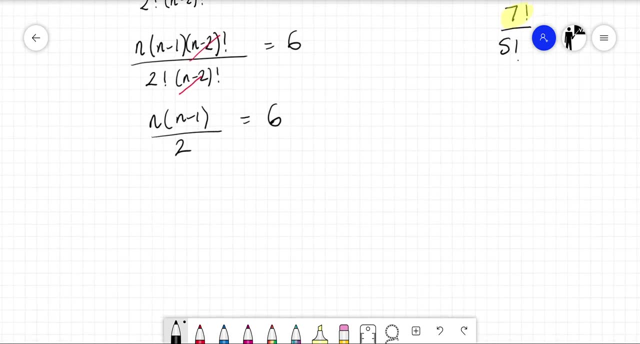 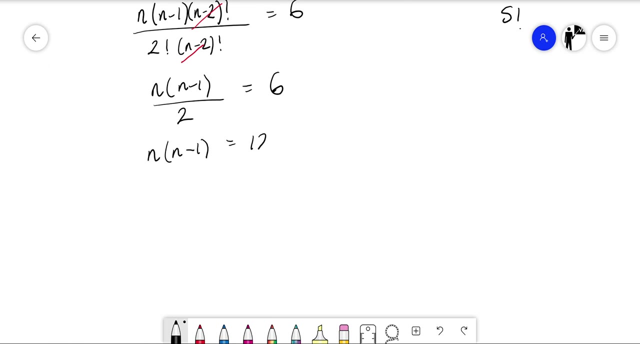 n minus 1 over 2 factorial. We can simplify our n minus 1 over 2 factorial, which is 2, which is equal to 6.. Now we're just going to hit and solve this n bracket. n minus 1 is equal to 12.. 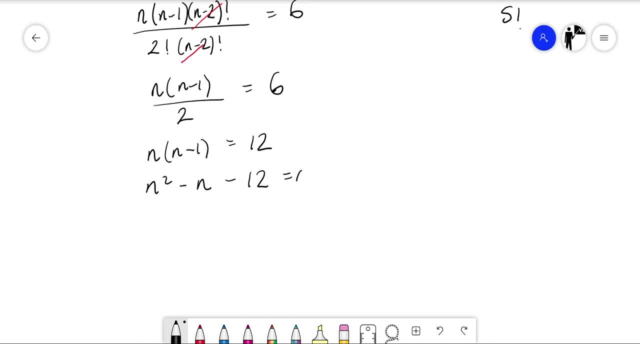 n squared minus n minus 12 equals 0. And if we factorize that we're going to have n minus 4, n plus 3 is equal to 0. We could split And we'll have n minus 4 equals 0. So we'll have n equals 4, and n plus 3 equals 0. So n equals. 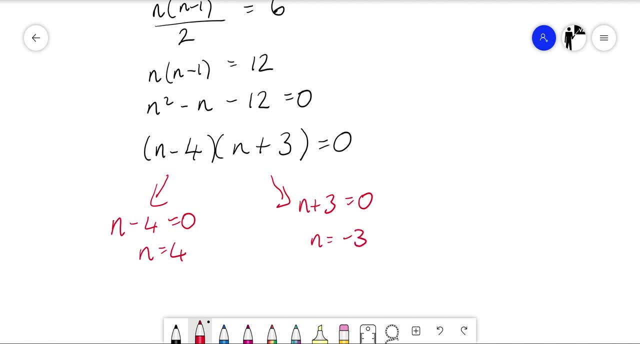 negative 3,. okay, But if we kind of link this to Pascal's triangle, remember this relates to the role that this would happen in, This relates to the role in which this would occur, And so, Pascal's triangle, we can only have positive rows or greater than or equal to 0,. 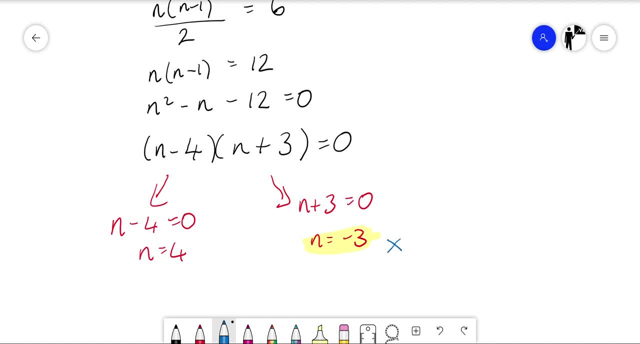 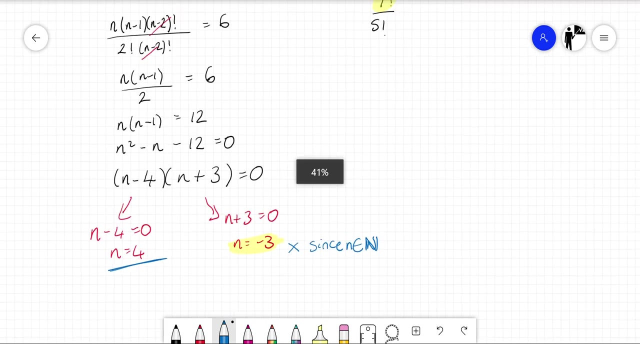 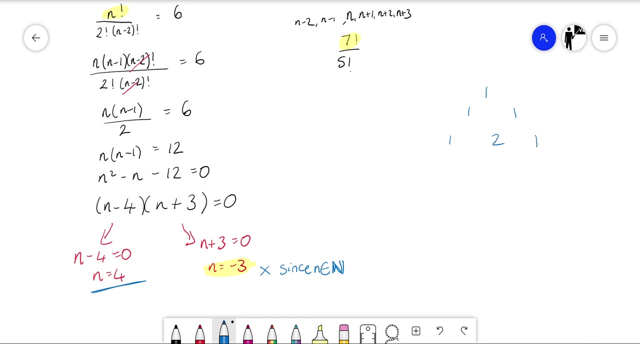 or rows. So this is not possible, since n has got to be a natural number. okay, So our answer here would be: n equals 4.. I'm just going to link this as to why this would be the case. I suppose you could have actually just went ahead and used Pascal's triangle to work this out. 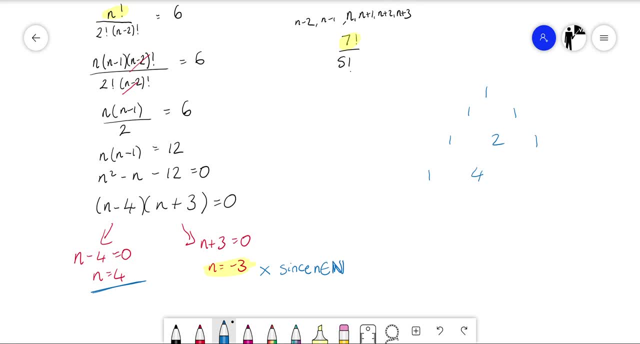 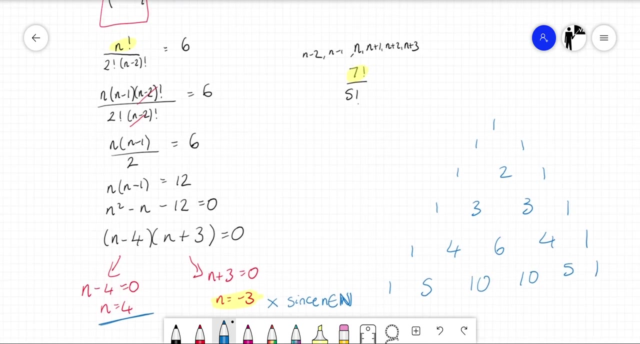 one four. oh, that's a mistake. one, three, three, one. I was going ahead to the next row there. One, four, six, four. one one, five, ten, ten, five, one. Okay, so we wanted to do something. 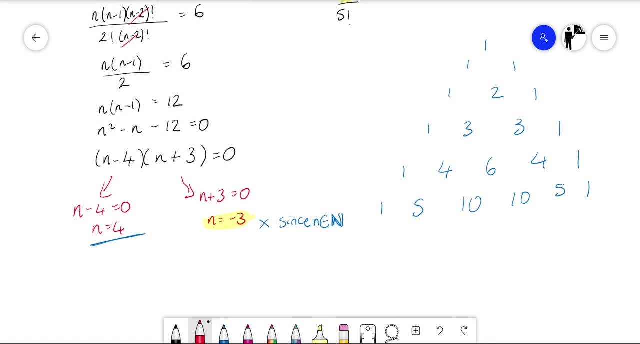 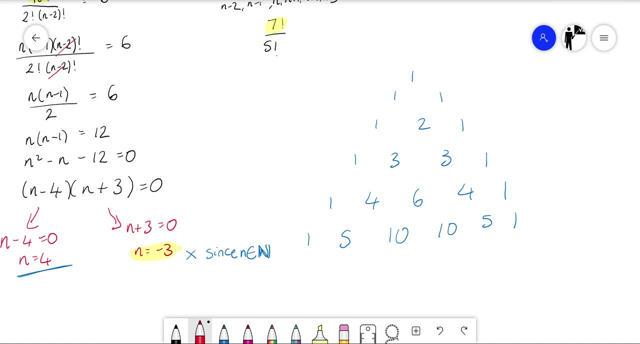 choose two is equal to six, So we could think about: okay, so in which options can I choose two? So that's zero, zero one, One, two. So that's the second element: Zero one, two. second element: Zero one, two, second. 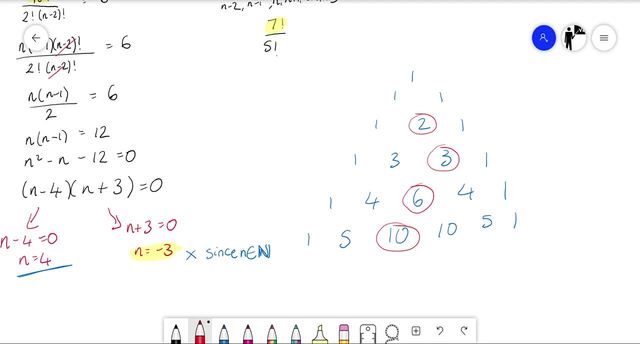 element Zero. one, two, second element: Okay, so then we can see here that we're working in row four. Therefore, n is equal to four. Okay, you could have gone that route, but obviously algebraically it's much more straightforward, particularly if it becomes a wee bit more. 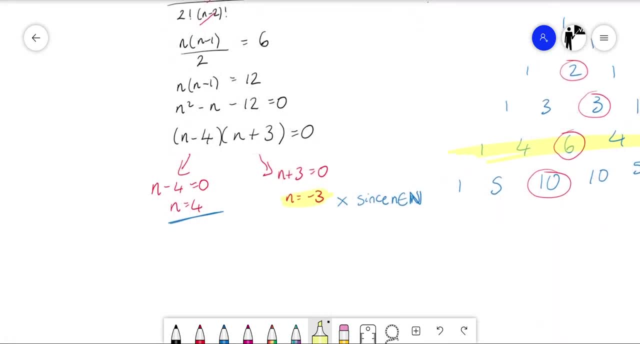 involved. Okay, that was example one. Example two: Let's do n choose one plus n choose two is equal to 28.. Okay, so this is a wee bit more awkward here. This is where we're going to need to draw upon this knowledge here from the previous video. 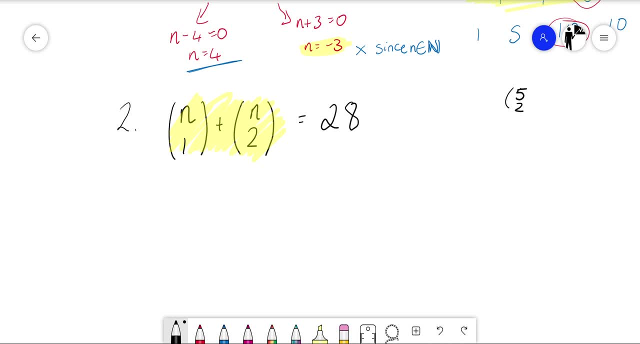 Remember before, when we had five choose two plus five choose three. The answer to that is no, So we're going to need to draw upon this knowledge here. from the previous video, The answer to that was 20, which is the same answer as six choose three. 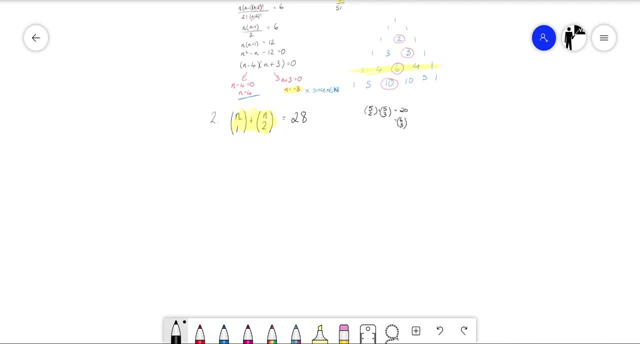 Okay, essentially. for example, we were in the sixth row. Oops, In the sixth row. to get this value here, we would add the two values below it. So notice what happens here. We essentially move down a row. Okay, so if we're moving down a row, 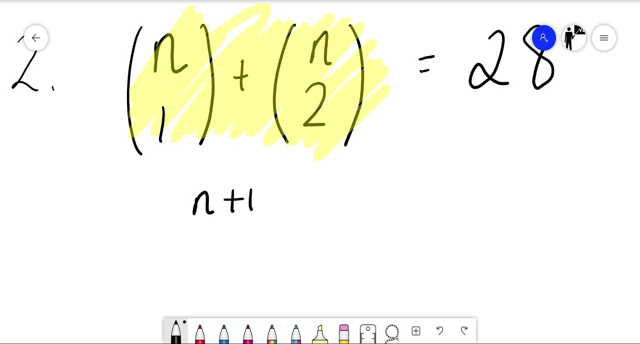 this would become n plus the nth plus one row. So if we started here at row two, if we were adding elements in row two, that would give us the result in row three, position two, and that's equal to 28.. 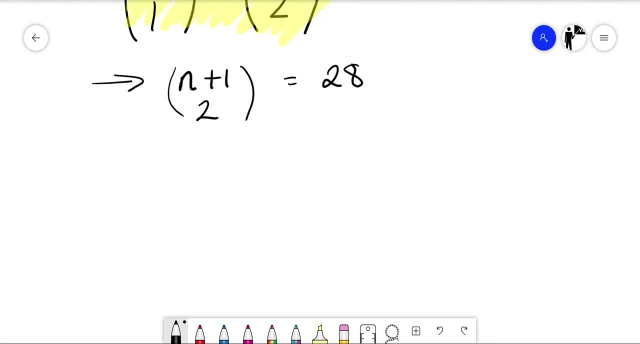 I'll zoom back a wee bit, So we are going to use our formula here, Remember. so n choose r. this is given to you in your formula sheet. is n factorial Over r factorial? n minus r factorial. Okay, so in this case n has been replaced with n plus one. 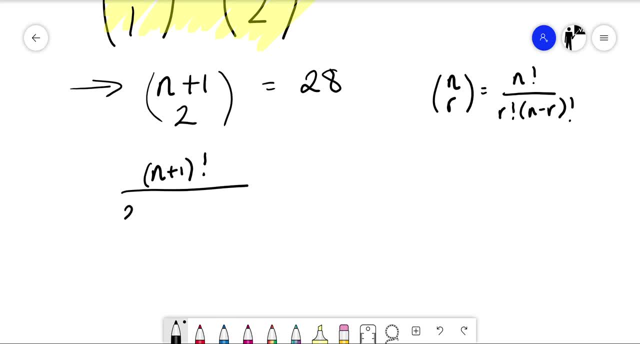 That's n plus one factorial over two factorial, n plus one minus two factorial, and that's equal to 28.. We can keep going ahead and solving here: n plus one factorial- that'll be a bit of simplifying first- Over two factorial, and that's going to be n minus one factorial, and that's equal to 28.. 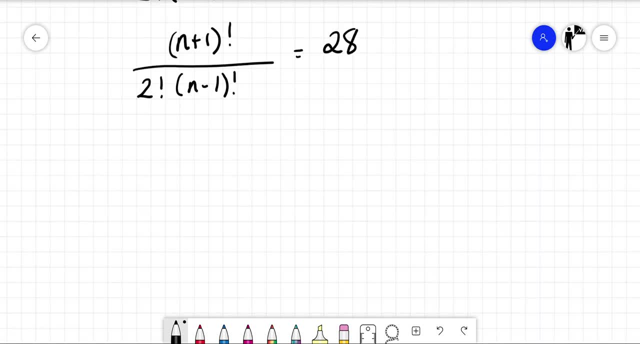 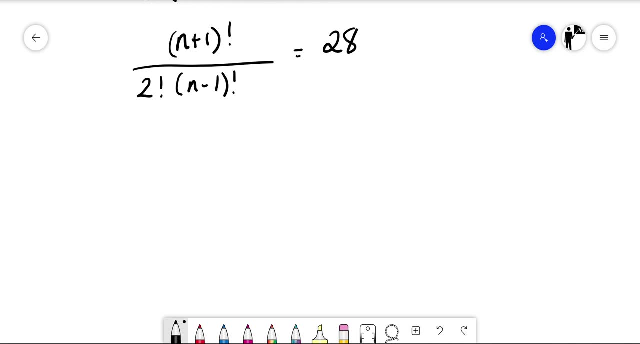 So we're going to want to simplify these factorials. So n plus one is bigger than n minus one. So we're going to rewrite n plus one factorial in terms of n minus one factorial. So n plus one factorial can be written as n plus one times n times n minus one factorial. 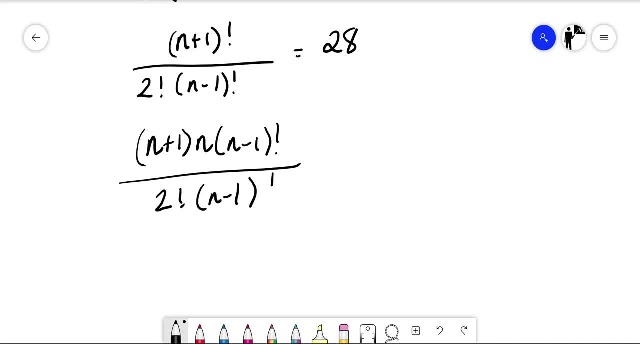 And that's over two factorial, n minus one factorial, and that is equal to 28.. We can simplify here And I'm just going to write it. So we've got n plus one times n. So I'm just going to write that as n bracket n plus one over two factorial, which is two. 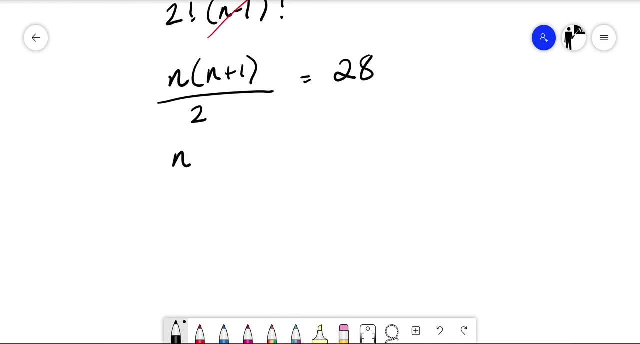 which is equal to 28.. And keep going and solving here Is equal to 56.. So we've got n squared plus n minus 56 is equal to zero, Which is going to factorize into n plus eight. n plus eight, n minus seven equals zero. 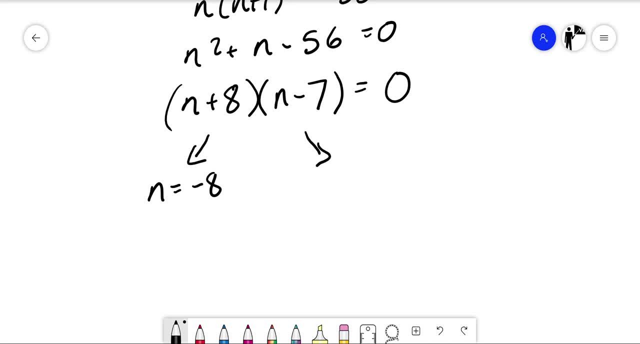 We can split and solve. n is going to be negative eight. n is going to be seven. It can't be negative eight. We can't have a negative eighth row. The values of n need to be greater than or equal to zero. 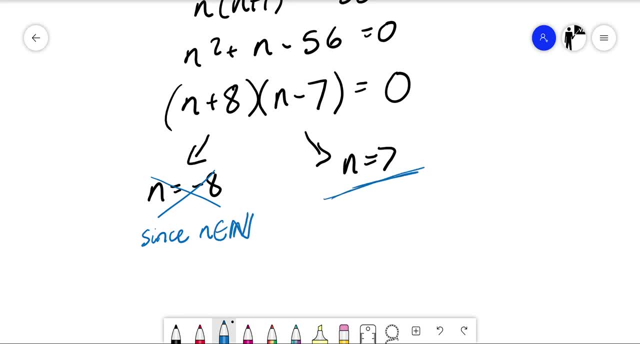 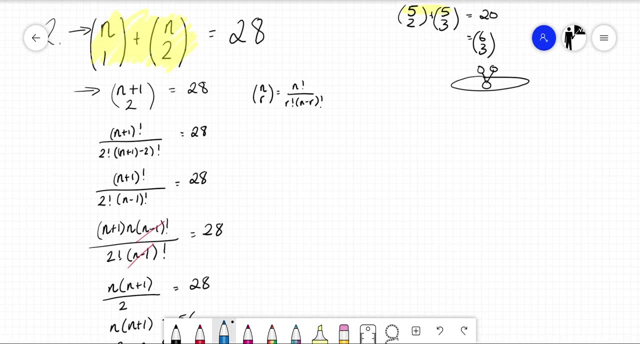 The values of n are natural, So therefore n is equal to seven. Okay, let's even just think about this in terms of Pascal's triangle again. You wouldn't be expected to do this, but I always like linking it back. 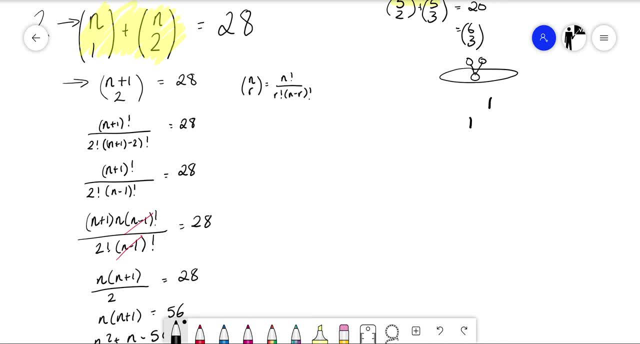 I'll try and make this as big as I can here. So we've got one one one one two, one one three, three, one one four, six, four, one one five, ten, ten, five, six, seven, eight. 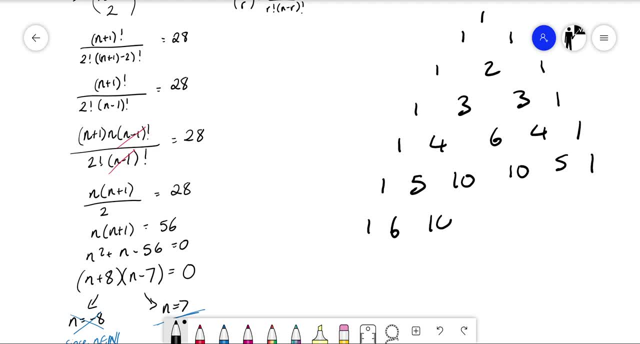 Ten five, One. And now we're at our seventh row here. I need to move that over a wee bit. One seven sixteen twenty. I made a wee error here. That'll be one six, fifteen twenty, fifteen six one. 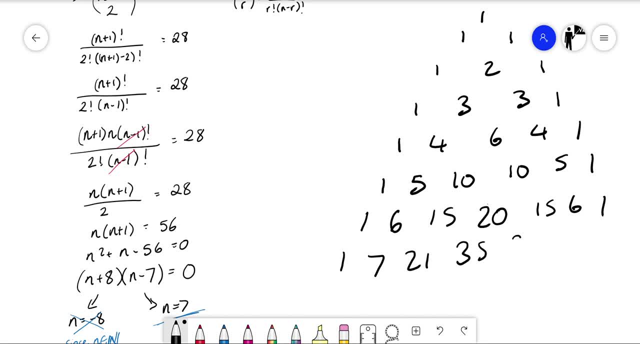 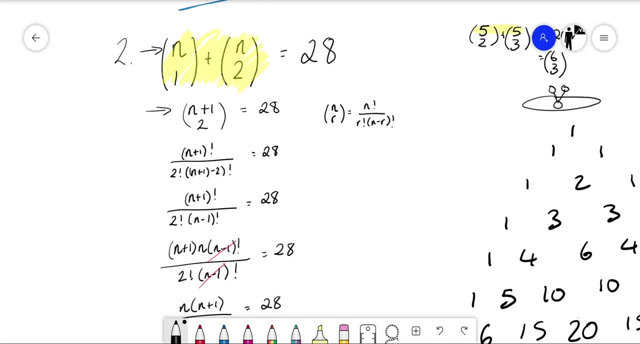 Then one, Seven, twenty one, thirty-five, thirty-five, twenty-one, seven, one. Okay, so we wanted to work out when, in Pascal's triangle, does it happen that when I add the first and the second element together, that I get twenty-eight? 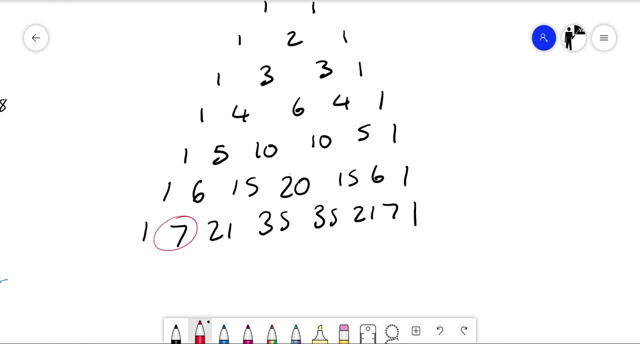 Okay, and we can see that in the seventh row here. when I add the first and the second element together, I get twenty-eight. So therefore n is equal to seven. Once again, you wouldn't be expected to do this. 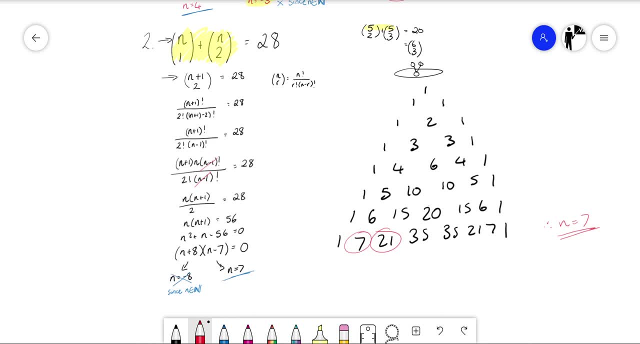 You wouldn't be expected to use Pascal's triangle, but I'd just kind of like to try and link it together. Thank you very much.